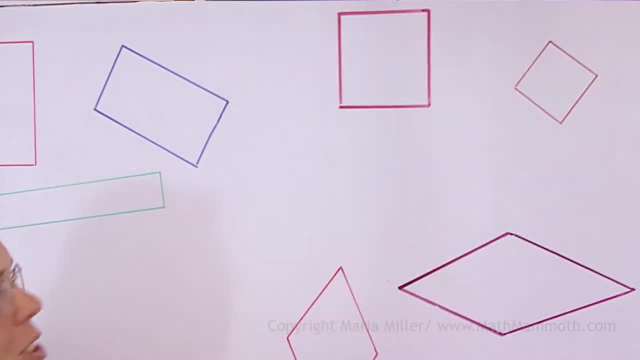 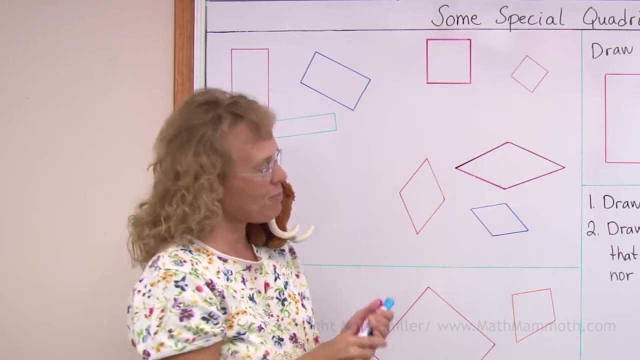 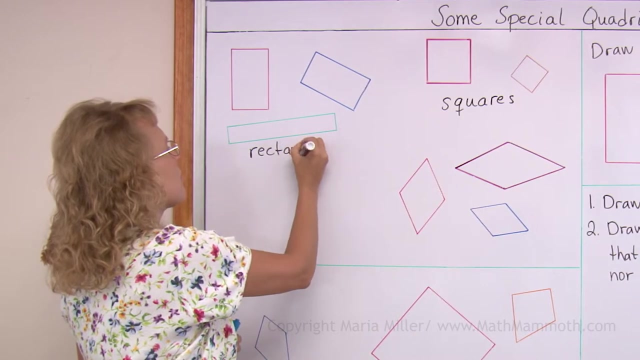 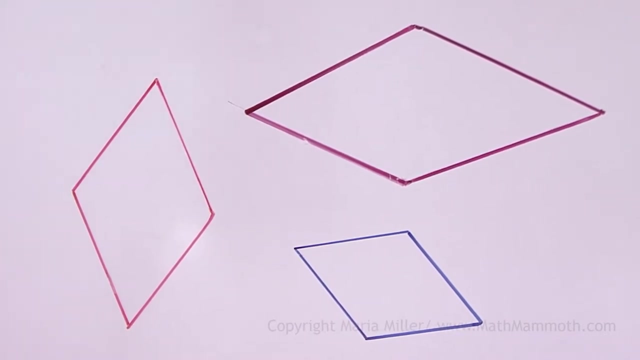 are rectangles because each of these corners also is like a straight corner, But additionally each side has the same rectangle. So let's write here squares and over here rectangles. But what about these? They are special quadrilaterals too. You probably have seen them, and they are usually called diamonds. 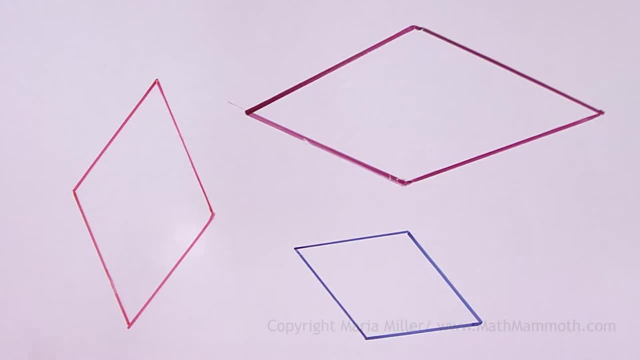 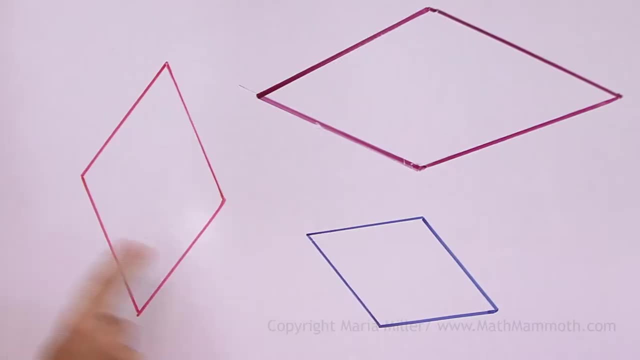 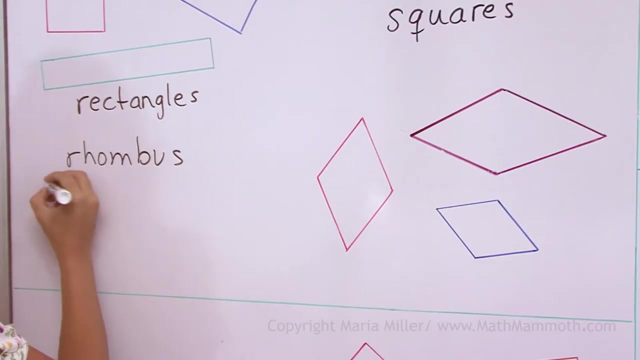 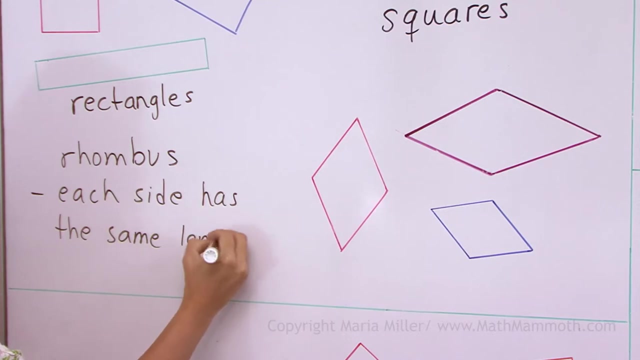 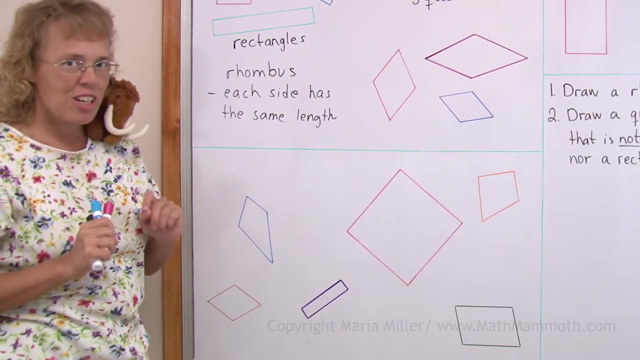 but in mathematics we have a different name for them. One of them is called a rhombus. many of them are called rhombi, And they are special because each side has the same length. So let's write here rhombus, and each side has the same length. So diamonds or rhombi Over here. Your task is to find. 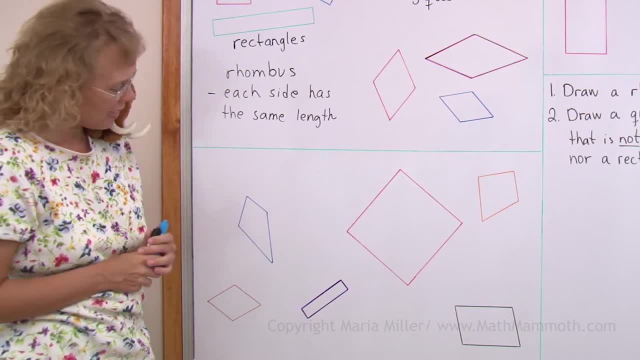 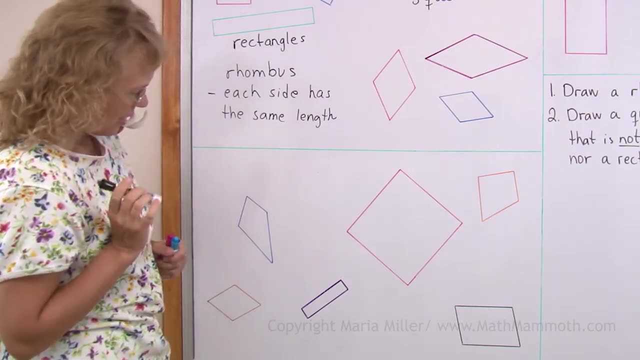 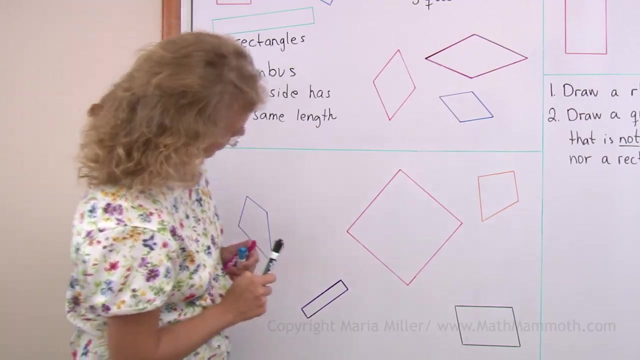 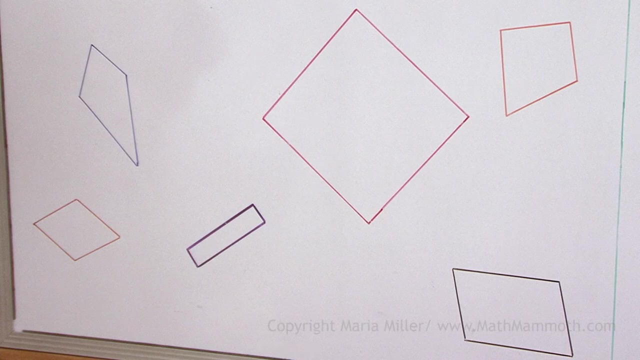 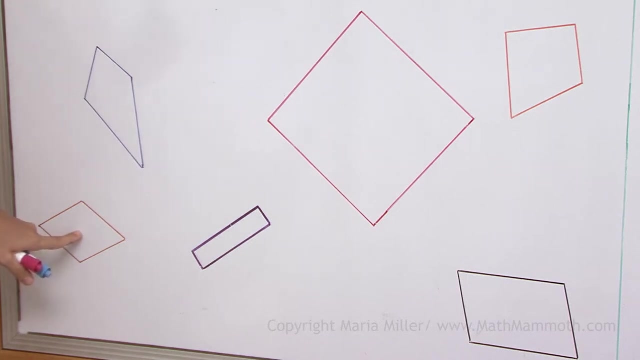 those special quadrilaterals and name them. Okay, I'm just gonna find any rectangles- Yep, this one is a rectangle. Any squares: This one is a square. And then any rhombi- Okay, there's just one, It's this one, Okay. Or a diamond. 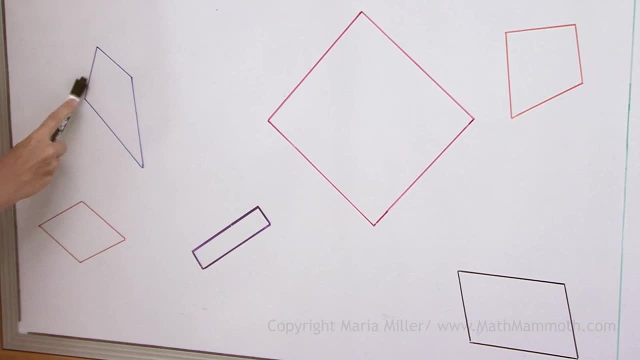 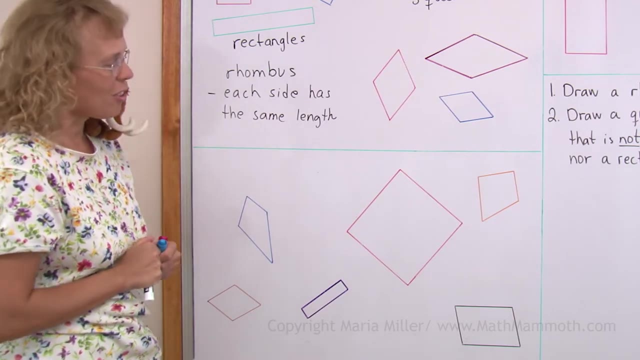 shape. This one is not, because each side is not the same length. Okay, shorter and longer, and so on. It looks kind of like a kite. That's another special quadrilateral. actually, This one is not anything special. Now, this one is actually another special kind. 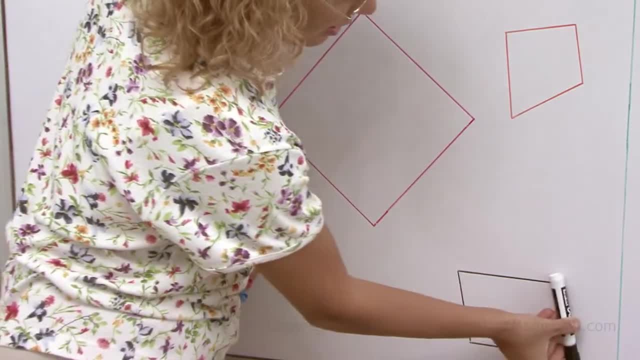 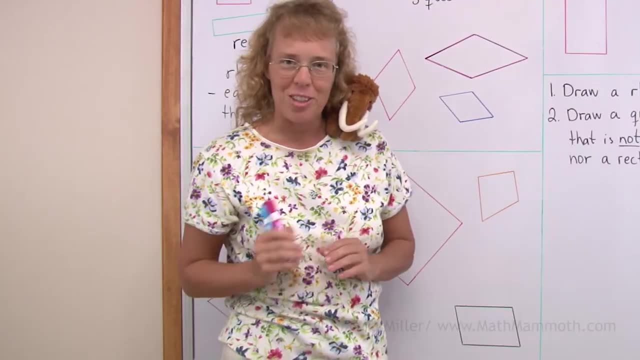 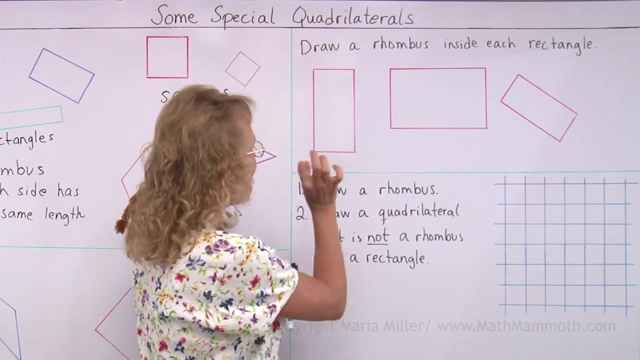 called a parallelogram because this and this side go towards the same direction. they're parallel, and also this and this side. Okay, let's go on, Draw a rhombus inside each rectangle. This is kind of neat, because inside each rectangle we can easily draw a rhombus, or 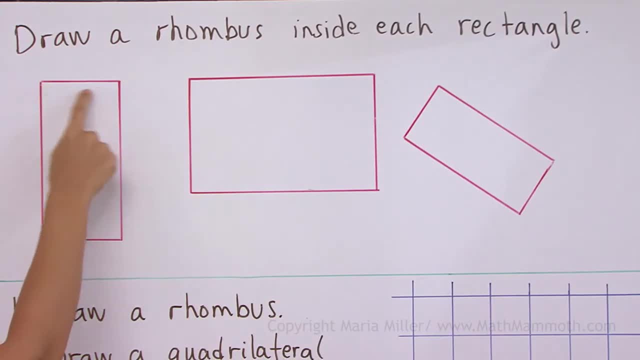 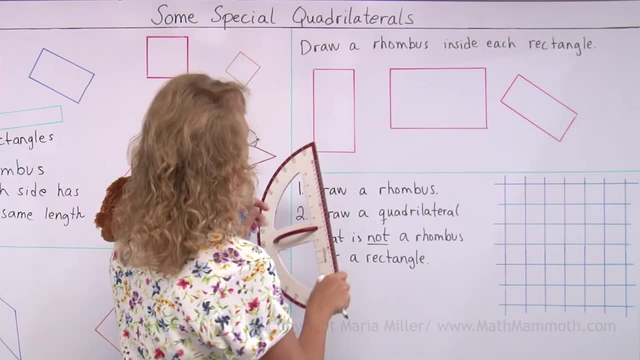 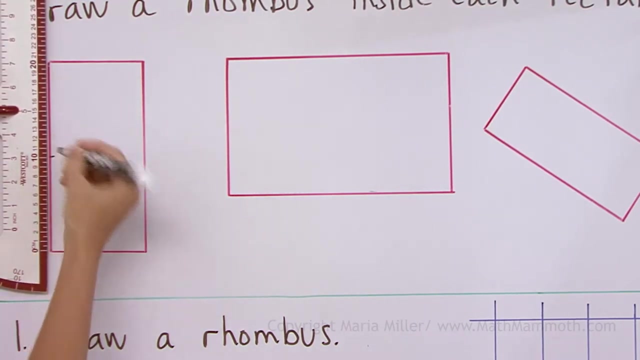 diamond shape, And all we need to do is find the midpoint, the exact middle of each side, and then connect the dots. And so let me measure here. Okay, this is 20 centimeters, so the midpoint is here 10.. 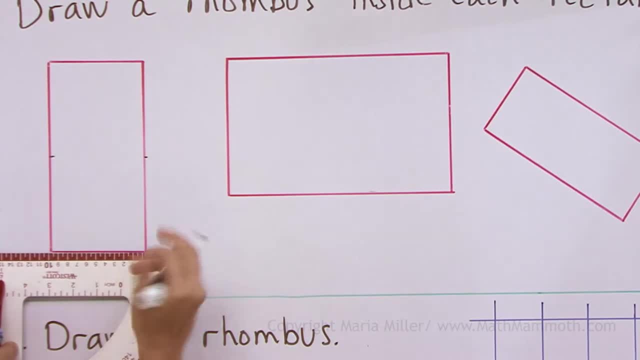 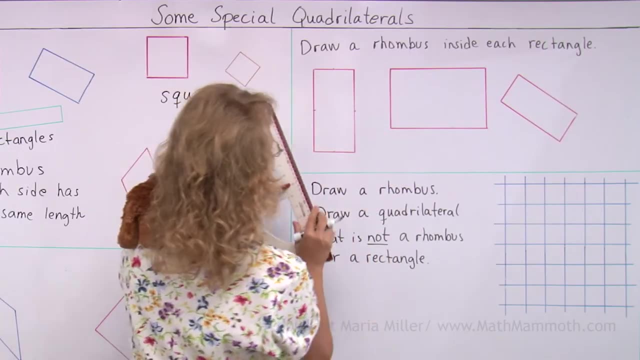 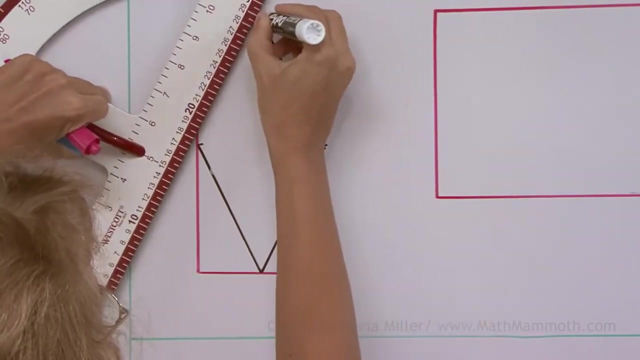 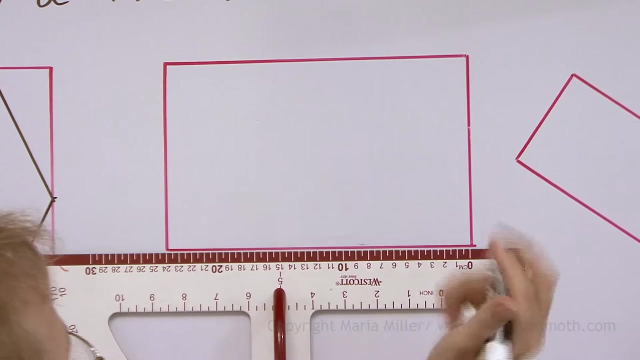 The same here. This is 10 centimeters, so the midpoint is at 5.. Okay, and now I just connect those There. a rhombus, Let's do the same here. 24 centimeters, so we have it here at 12.. 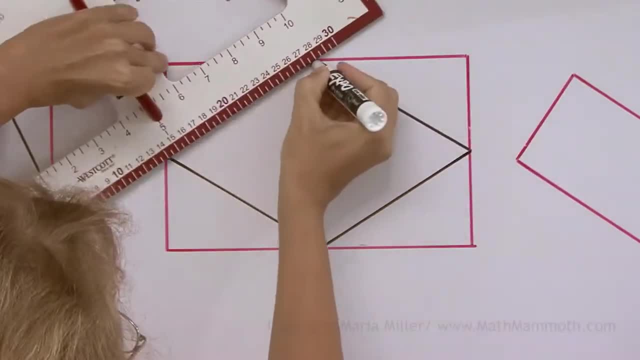 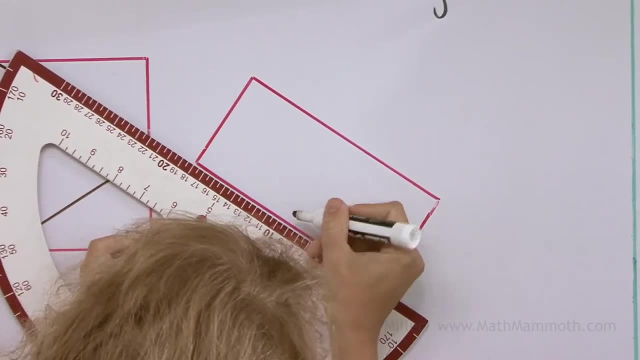 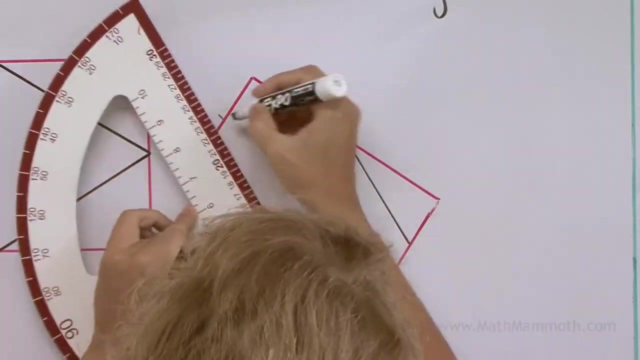 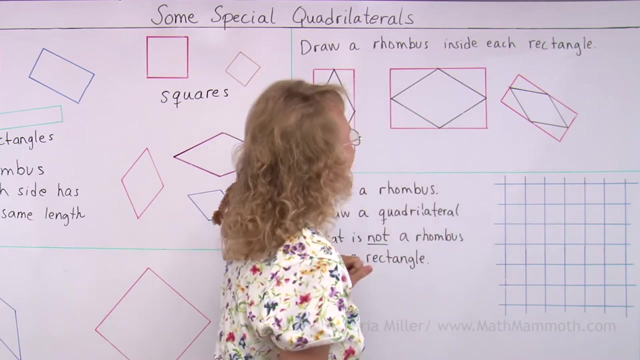 It's a pretty solid rhombus. Okay, do you like that one? And then the last one. And here's my last one, And you can try this method too, at home or at school. Just draw some rectangles and then you are done. 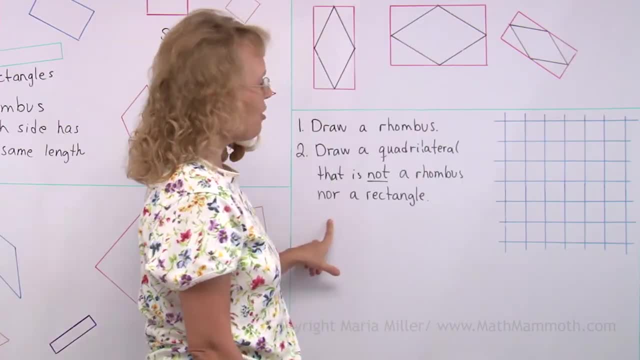 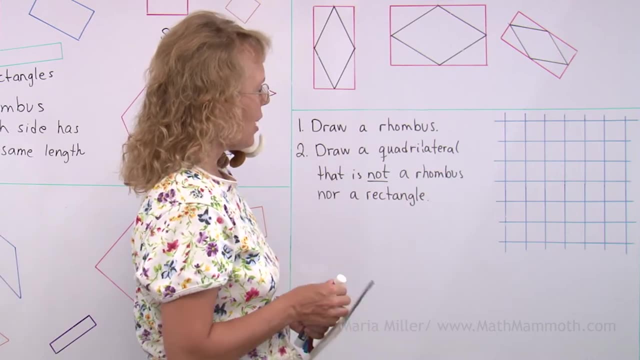 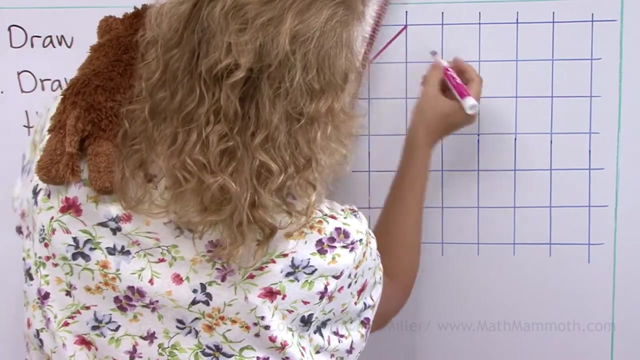 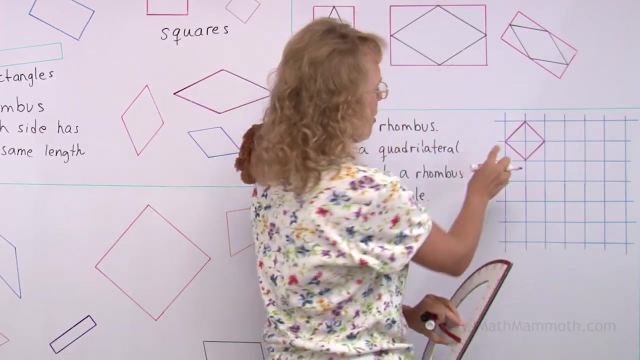 then, inside them, draw some rhombi. Now, over here I have a grid and we need to draw a rhombus first of all, and there's many ways to do that. I could, for example, go like that: Okay, that actually is a square too. Now is a square, a rhombus- Yes. 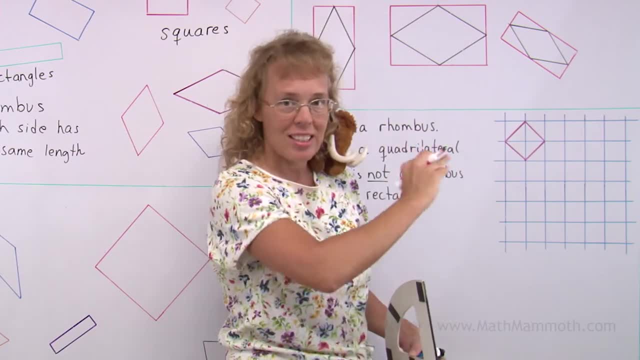 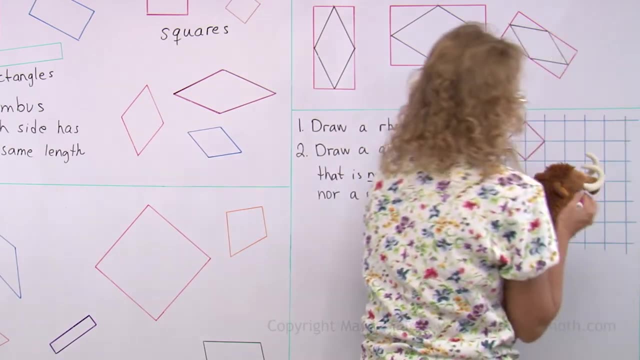 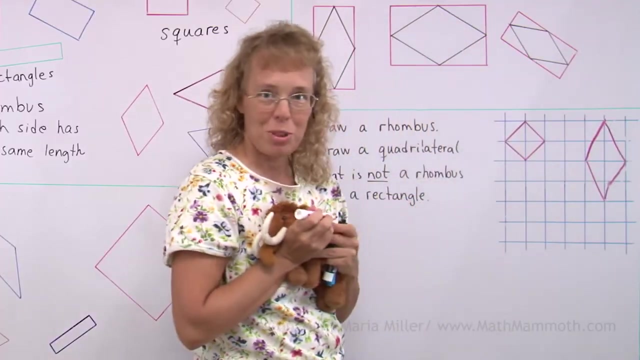 it is because in a square you also have four sides that are the same length. I'll draw another one. Oh, okay, Matthew wants to draw. Okay, come on, You want to draw one. So there's another rhombus by Matthew. Draw a quadrilateral. that is not a. 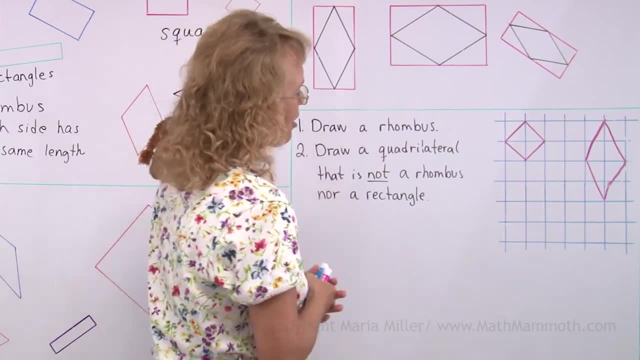 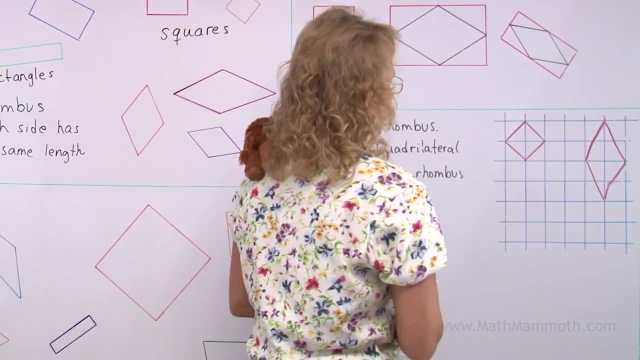 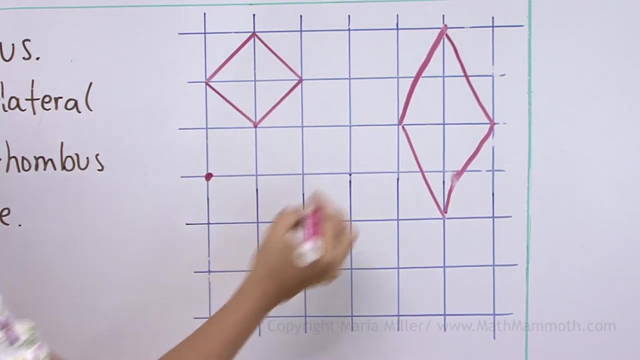 rhombus nor a rectangle. Of course, it would be easy to draw rectangles here, right, Like this: All right, Okay, Or this or this. So draw something that's not a rectangle and not a rhombus. Now, if I use these grid points as my vertices, then let me see, for example, These four: